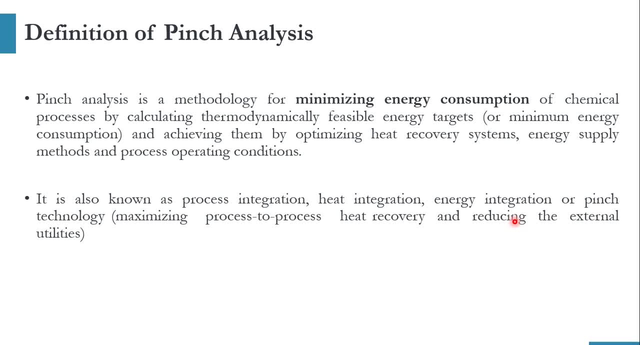 So the pinch analysis? why it is used? what is the definition of pinch analysis? Pinch analysis is a methodology using which we can minimize the energy consumption of a chemical plant or a process by calculating thermodynamically feasible energy targets or minimum energy consumption. 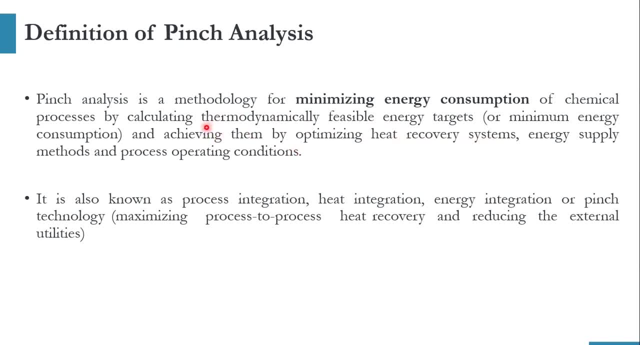 and achieving them by optimizing heat recovery system, energy supply methods and process operating conditions. Basically, this is a technique In which we optimize the system. we increase the efficiency of the system. How we can increase is obviously in a process. we require the utilities, like heating utilities. 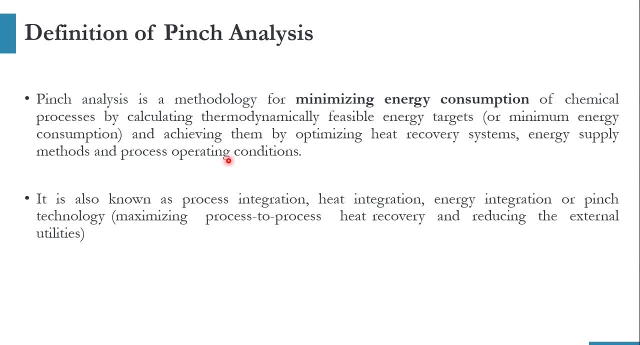 we require steam, furnace oil and different heating utilities and same for cooling utilities, like we require cooling water, air and so on. So basically, if we reduce the utility requirements, this is one step of increasing the efficiency or energy efficiency. You can say decreasing the cost, minimizing the energy consumption, or, if we can heat, integrate. 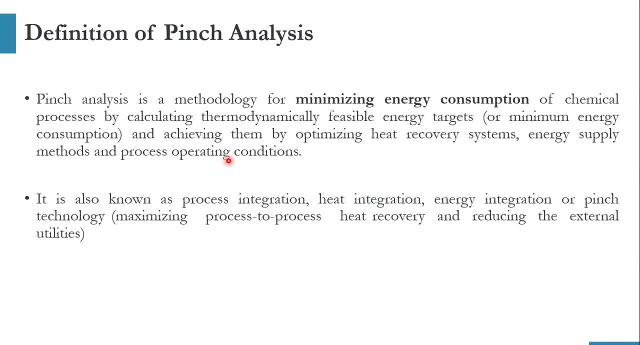 For example, for a distillation column you need a heating utility in re-boiler and a cooling utility in condenser. But if somehow we can integrate a column with a source which provides the cooling utility or partial cooling utility or provides a partial heating utility, then what happens? 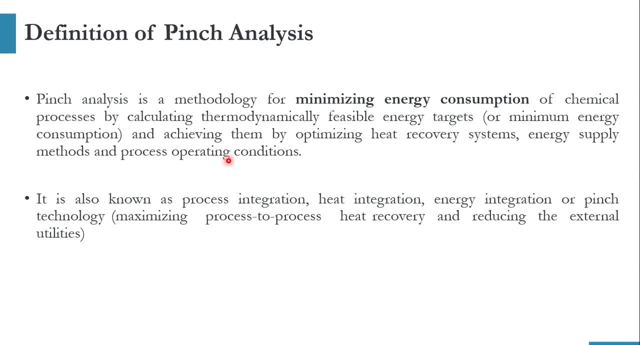 The steam requirement will decrease. the water requirement will decrease. How we can do it, like we can preheat the field to decrease the utilities requirement. So there are different methods by which we can optimize the system. likewise, We can decrease the energy consumption and how we can do it. 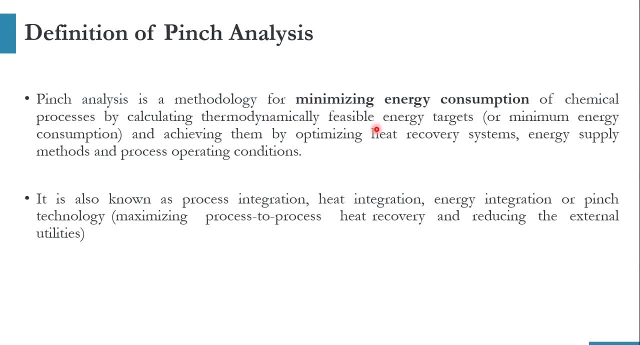 By some energy targets which are feasible energy targets. Obviously, we have to talk about some practical targets. in practical targets it is also known as the process integration, heat integration, energy integration or pinch technology. in other words, it could be said that maximizing process to process. 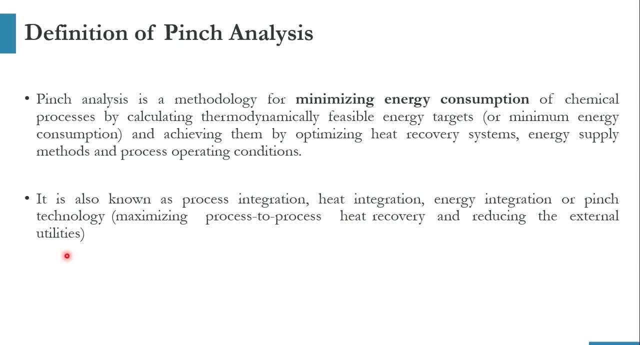 heat recovery and reducing the external utilities. what are external utilities? again, i have told you: steam cooling water and so on. for example, if there is a process a which is releasing energy and it is going to the atmosphere and wasting, and for process b, you require energy, what you can do: 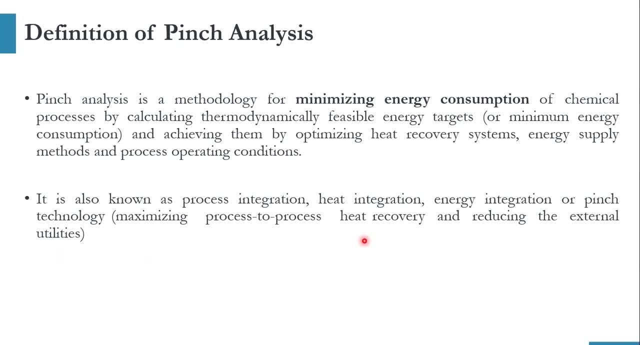 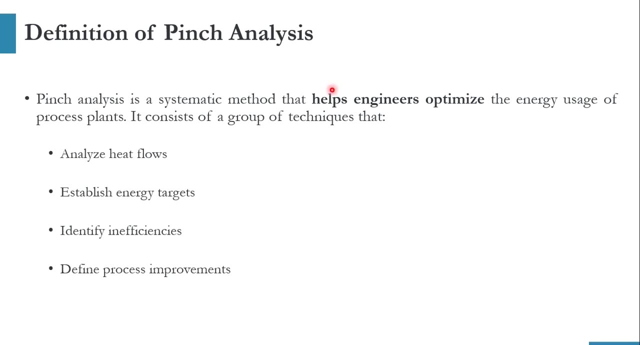 you can integrate both process a and process b to minimize the energy consumption, which is the external utility consumption, and you can optimize the whole system. it is a systematic method which help engineers optimize the system and optimize the energy usage of process plants. what it involves? analyze the heat flows. first thing you need to do that. you have to analyze the current heat. 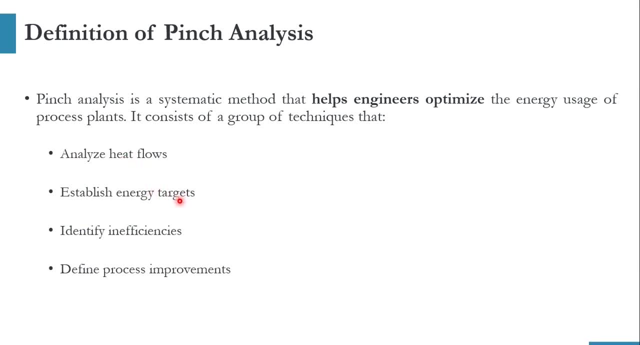 requirement of the system. then you have to develop the energy targets, that how much reduction you require, percentage of reduction: we will see in upcoming slides that we require some percentage recovery of the system or personalized reduction in the cost of the system. then identify the inefficiencies. obviously you need to identify. 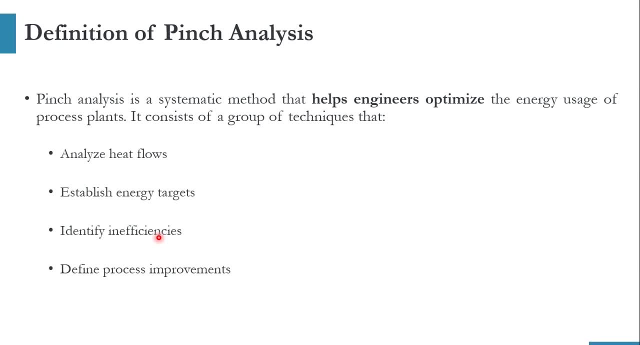 where the heat is leaking. for example, if in case of boiler you need to identify the part where there is a maximum heat loss, obviously if you install the insulation at that part, obviously you can save energy and again define process improvements. so, first thing, analysis of the system, then 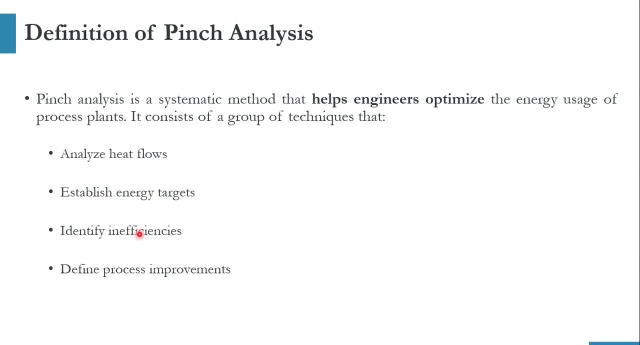 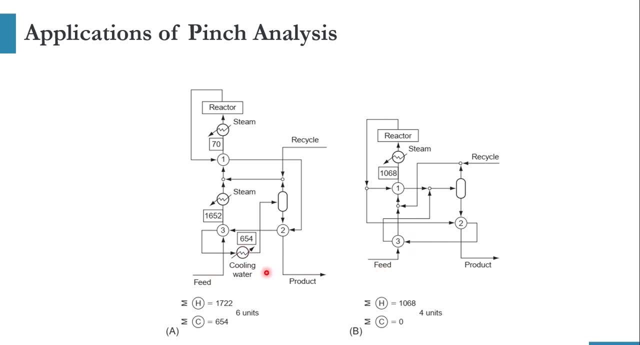 setting some target, then identifying the inefficiencies and then suggesting the process improvements. now, if you look at these two systems, first you look at this system, which is the number one field is going to number three, which is the heat exchanger. then this exchanger, where utility is required, 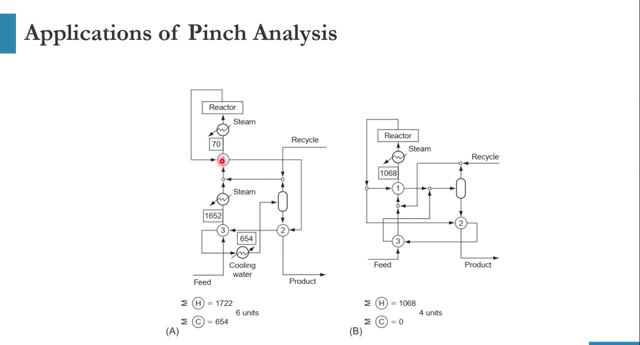 which is steam mixing with the air. one again steam requirement going to reactor, coming back here, exchanging heat, going here and this loop goes, then cooling water requirement and then. so this is the overall loop and for this system you can see that the total heat required summation of h is 172 to kilowatt, while summation 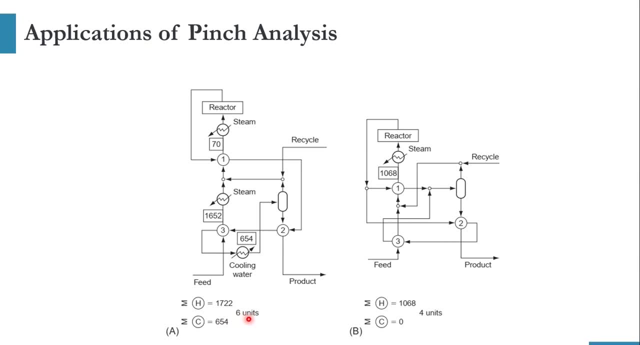 of c is 654 and there are six units required for this process, as you can see: one, two, three, four, five and six, so six units. total heating and utility requirement is one, seven, double two. total cooling requirement is 654 kilowatt. now, if you look at this improved system, 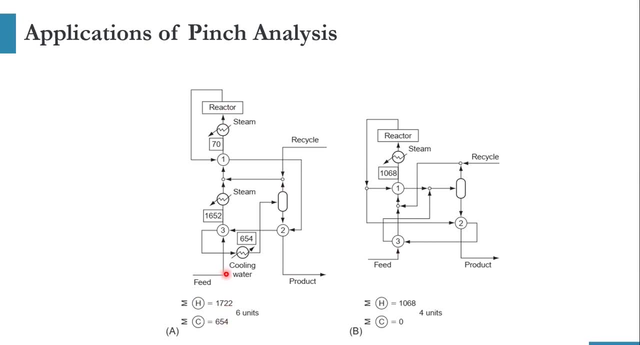 first you have identified or analyzed the heat flows. now your task is: for example, you have to decrease the utility requirement by a 10, then you will see that, what type of improvements you can get and how, by identifying the inefficiencies. so once you have shifted to this system, 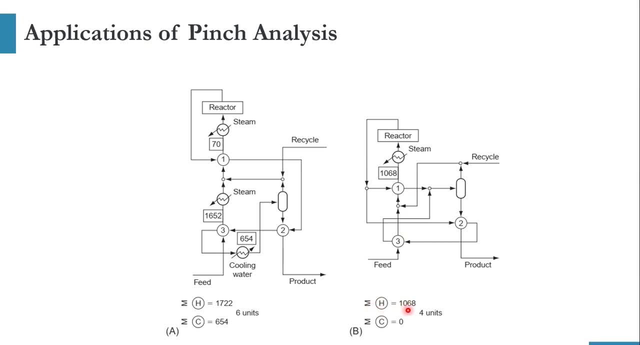 i will brief it like this: that the heat requirement or the heating utility requirement have decreased to 1068 kilowatt- from 172 to kilowatt and there is no cooling requirement means cooling water flow rate is zero. and this system- there is no requirement of cooling water. 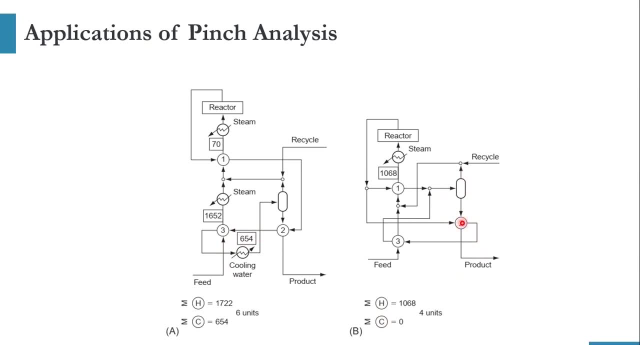 in this improved system. and now, instead of two heat exchanger for steam, there is only one exchanger for the steam and, as you can see, there are now four units. so you have saved two units of heat and you have saved heating utility. you have completely eliminated the cooling utility. 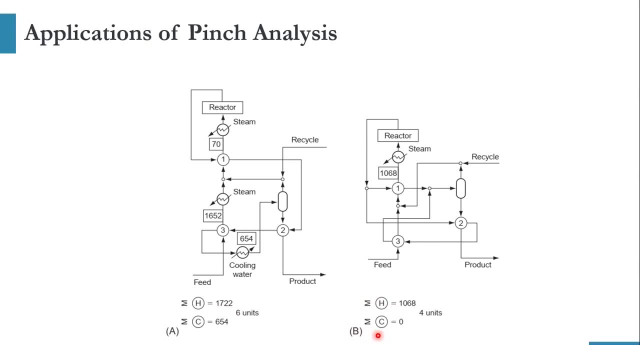 requirement. so that is how pinch analysis work, that it has optimized the system, how, by analyzing the heat flow, setting the energy targets, identifying the inefficiencies and doing the process optimization- earlier for the feed heating utility was used, but now, by improving the process to process heat recovery, the system is improved. so you can see that the system is now improved. so you 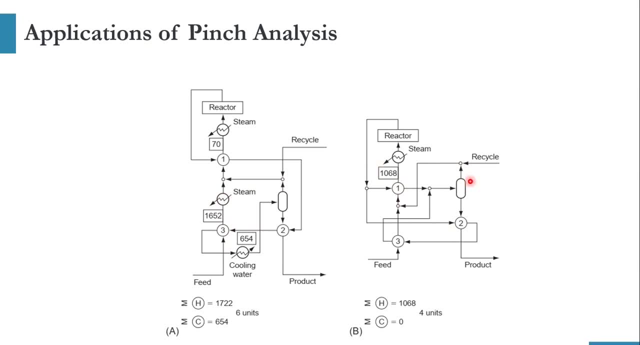 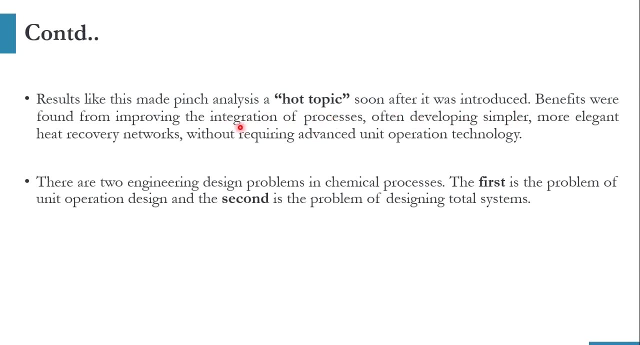 can pause it over here. look at the system and you will understand that how it is happening. results like this made pinch analysis a hot topic after it was introduced. benefits were found from improving the integration of process, often developing simpler, more elegant heat recovery networks without requiring advanced operation technology. remember, there are always two engineering problems. 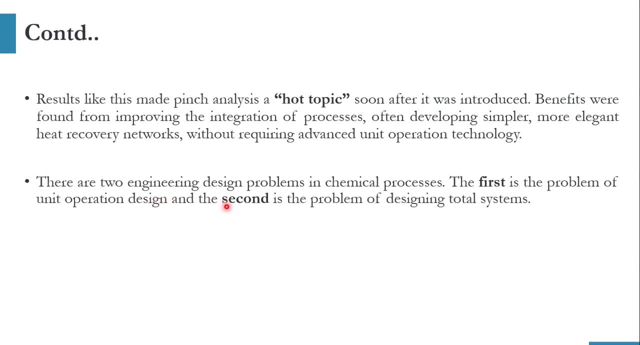 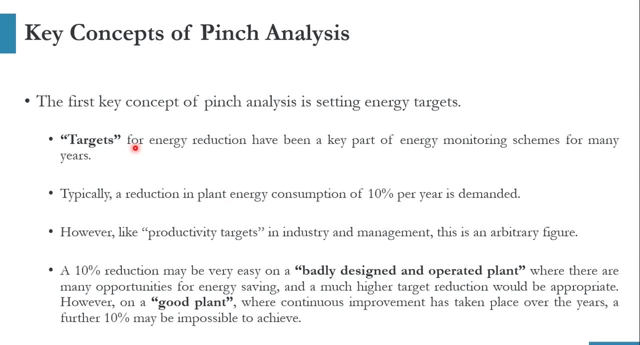 in chemical process. first one is related to the design of a single equipment and then designing the whole system. now we have been continuously talking about the targets, targets. what are the targets? basically the target for energy reduction: that how much reduction we required typically in a chemical process. increase in energy consumption of 10 percent per year is demanded. 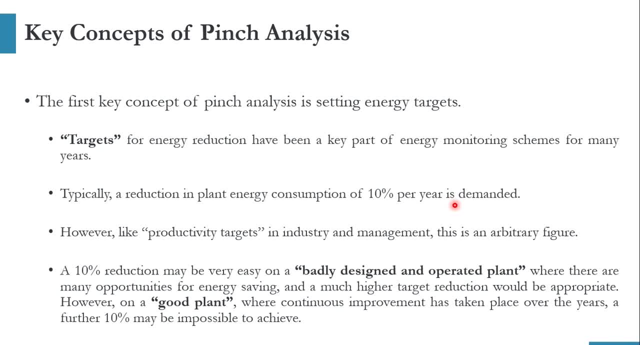 and that is quite achievable in a badly designed plant and badly operated plant. if a plant has more heat losses and it is quite inefficient, then you can achieve 10 percent more than 10 percent over there. but if a plant is designed perfectly or you can say: is a, it's a. 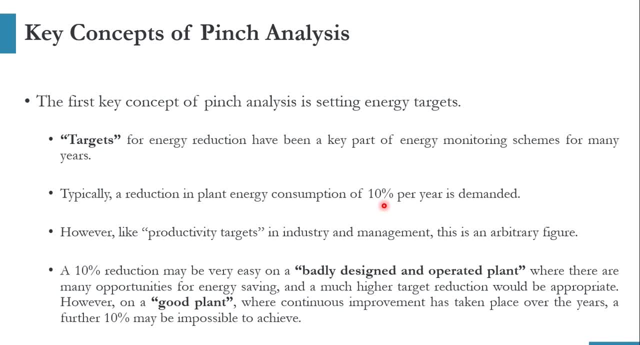 good design and it has been operated in a good way, then this target is quite hard to achieve. typically, a reduction in plant energy consumption of 10 percent per year is demanded. however, like productivity targets, this is an arbitrary figure. it could increase and it could decrease, but there 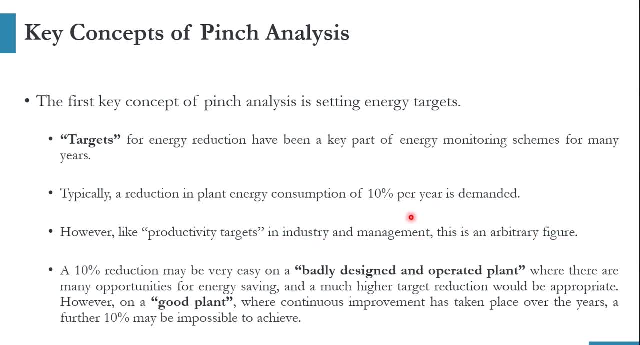 is some value which is available in the literature of 10 percent. a 10 percent reduction may be very easy on badly designed and operated plant where there are many opportunities for energy saving, and a much higher target reduction, which is 10 percent even. you can go to 20 and so on, which one is visible and that scenario, however, on a good plant where continuous 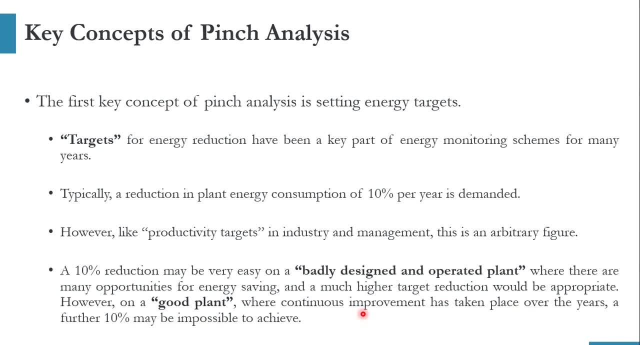 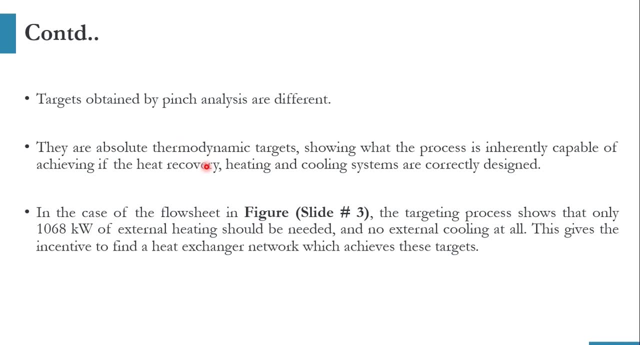 improvement has taken place over the years. a further 10 percent may be impossible to achieve again. this is the same information which is given in our previous slide, where we have studied the two. systems was decreased and cooling requirement was completely zero. Targets operated by pinch analysis are different. 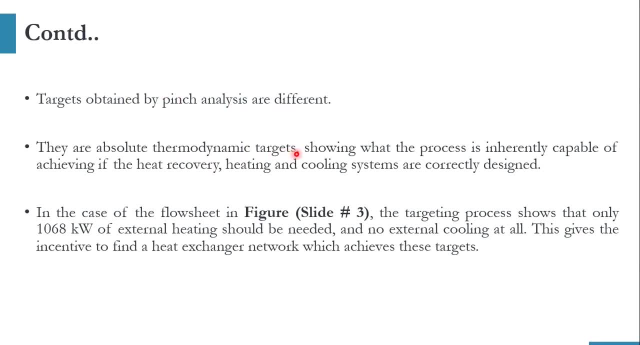 They are absolutely thermodynamic targets. Obviously, it should be thermodynamically feasible. How, Therefore? if you are talking about a heat exchanger, there should not be a temperature cross. This shows the feasibility. If there is a temperature cross that heat exchanger, you cannot install that heat exchanger. 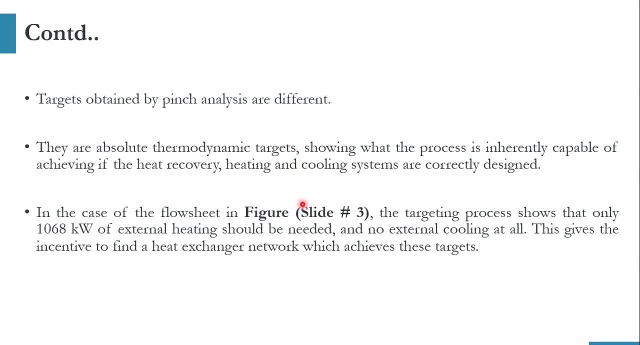 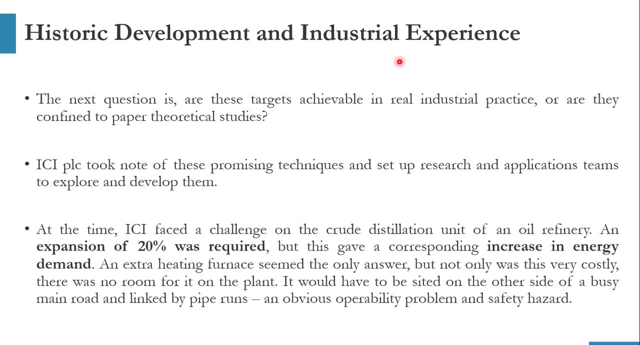 The size requirement and there are different things involved in it. Now, what is the historic development and industrial experience? It should be in your mind, or might be in your mind, that if this pinch analysis has some industrial applicability or not, Or is it just like a theoretical knowledge? 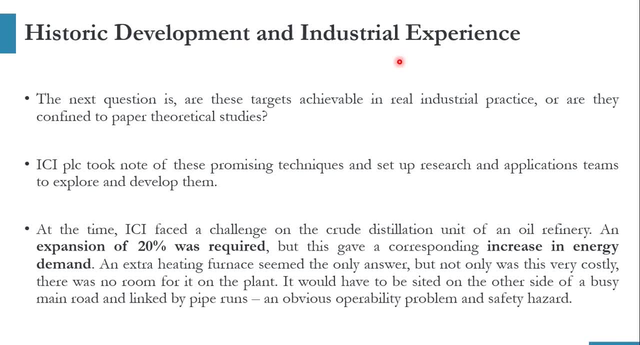 No, it is not a theoretical knowledge, but it has some industrial background. Around 90s, in 90s, ICI plant thought of expanding this infrastructure And for this you can write this paragraph Meanwhile, at the time, 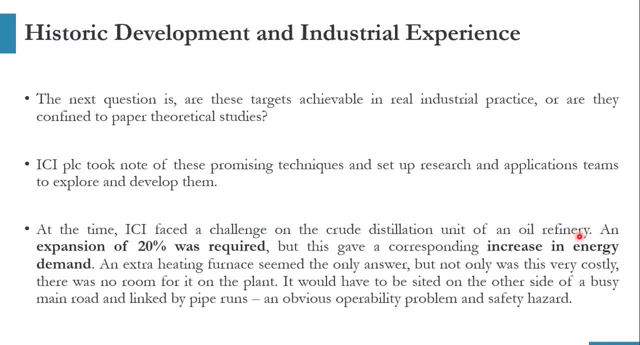 ICI plant thought of expanding this infrastructure, For this ICI faced a challenge on the crude distillation unit of an oil refinery. They wanted an expansion of 20%, But however, for this expansion of 20% they required a furnace. 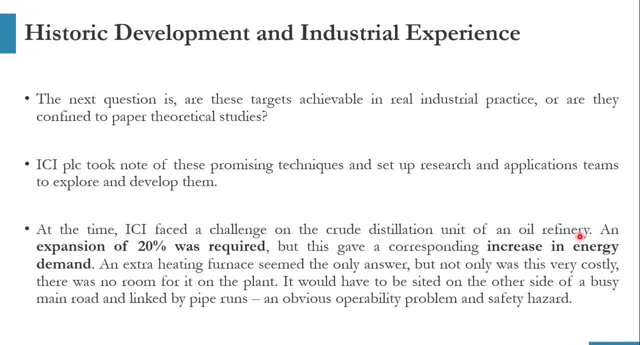 When they examined their facility, there was no room or no space for installing that furnace. It means that furnace needs to be installed not in the plant premises but outside the plant premises, And obviously not on the same road but opposite of the road. 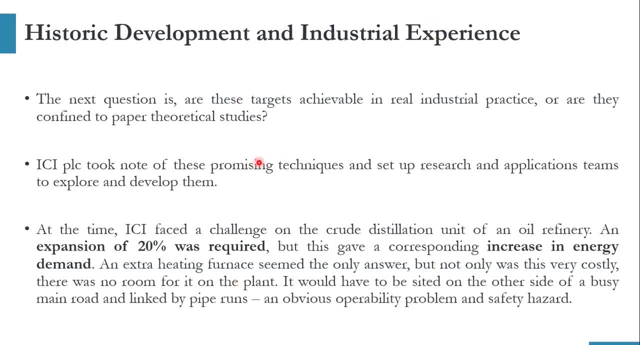 means the vehicles are passing through here, the vehicles are passing through here and one unit is installed over here, then the pipelines above goes to here. so that means a huge investment of pipelines, of infrastructure, to get the 20 percent expansion. and not only this, but there is a safety risk and 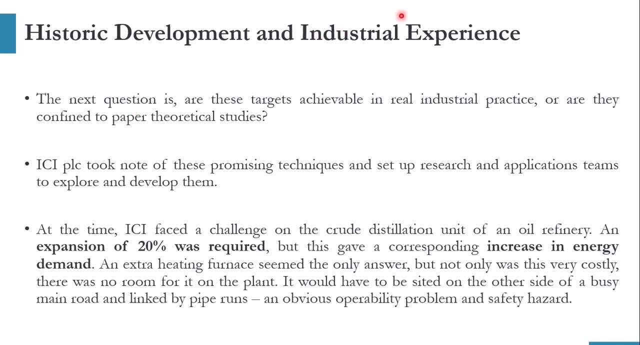 you know very well that if a line can explode or it can corrode or some issue or insulation may break, and different reasons as well, so what they need to do. obviously that solution was not practical. let me read it for you: that an expansion of 20 percent was required, but this gave an. 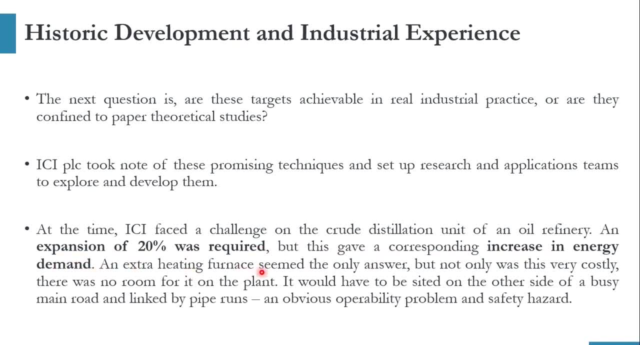 a corresponding increase in energy demand. an extra heating furnace seemed the only answer for this, but not only: this was very costly. there was no room for it on the plant and it would have to be sited on the other side of a busy main road and linked by. 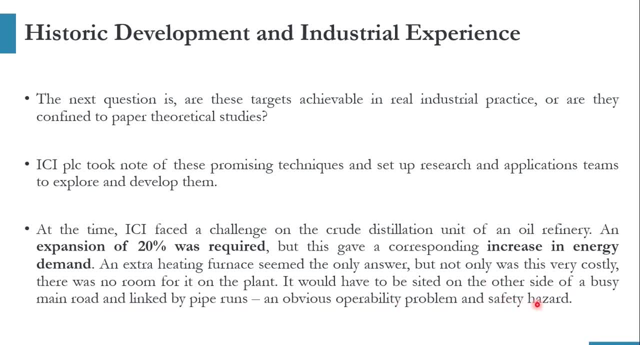 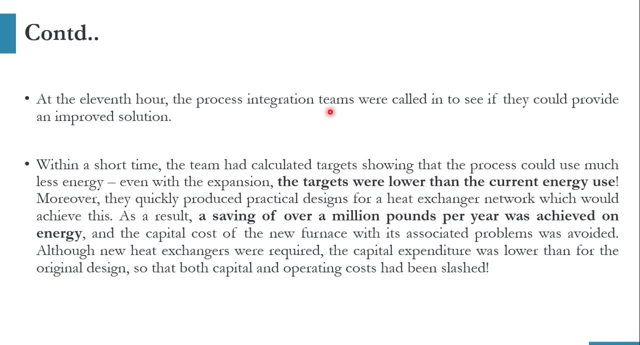 an obvious operability problem and safety hazard. so what they did? they called the team of experts, which is the process integration team, and within a short time the team had calculated the target, showing that even in the current system there is a full margin of improvement. that with this, 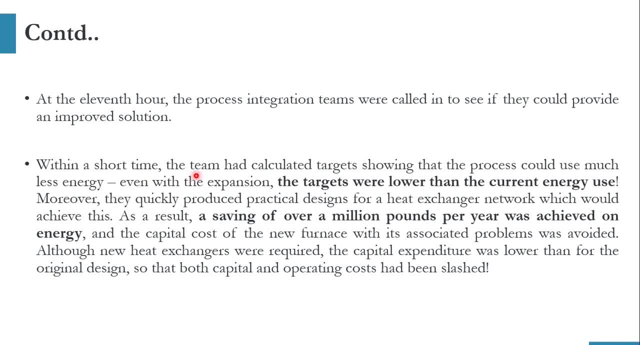 your energy requirement could have been reduced, but that within a short time the team had calculated target showing that the process could use much less energy, even with the expansion, that the furnace requirement was eliminated and even within the process you can extract the heat for your expansion. the target was lower than the current energy use and for this they have designed. 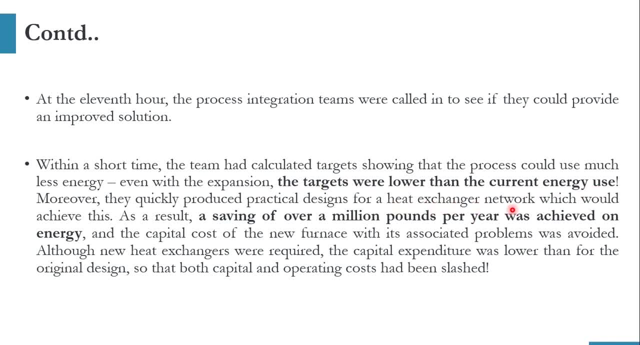 a heat exchanger network and a million of million pounds per year were saved, for this problem means- let me summarize it- that first, i see i need to expand the system by 20 percent. for this they required a furnace for it. they have designed that they required a furnace, but they did not. 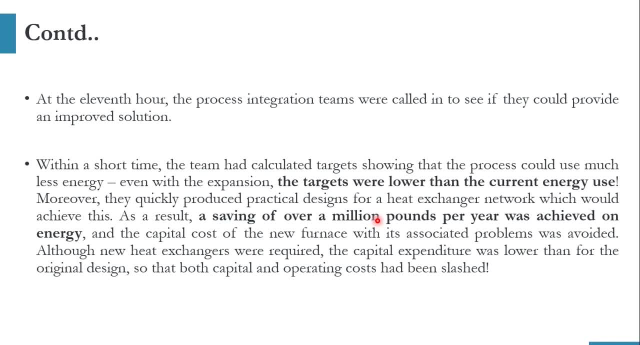 have enough space for it on the plant, they have to install it on the other side of the road. so what they did, they called the team. the team calculated the energy targets, the calculated the energy consumption of the plant and obviously they have step calculated all the steps to analyze the heat. 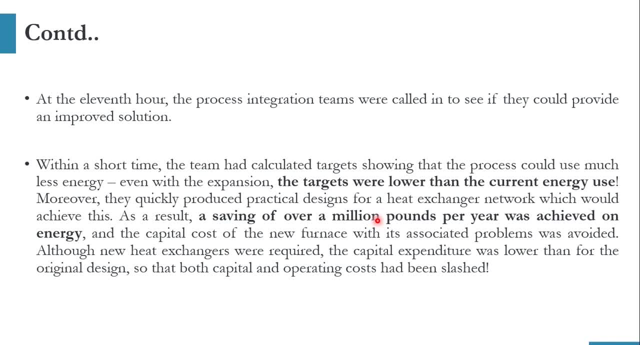 flows, then set the energy targets, then identify the processing efficiencies and process improvement. so when they have followed all the four steps, they came to the conclusion that even there was no requirement of the furnace and within a short time they had calculated the energy consumption within the system. there was so much margin of improvement that you can even extract energy. 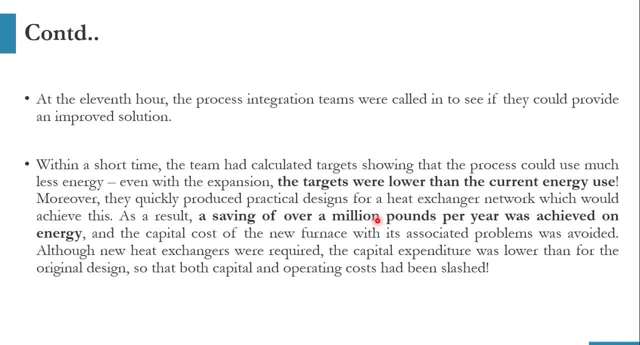 from process to process and a heat exchanger network was designed over here which was even saved million pounds per year in this system and you can see the capital cost of new furnace with associated problems were avoided. yes, there were new heat exchangers required, but obviously in 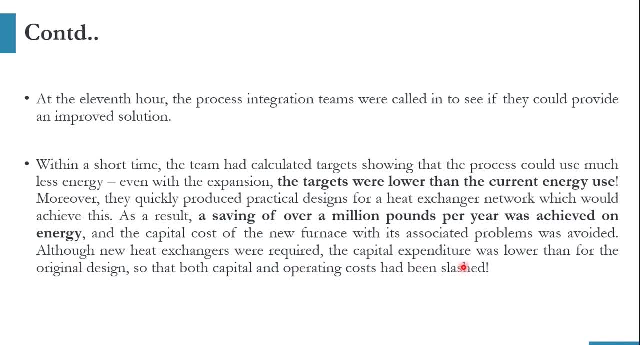 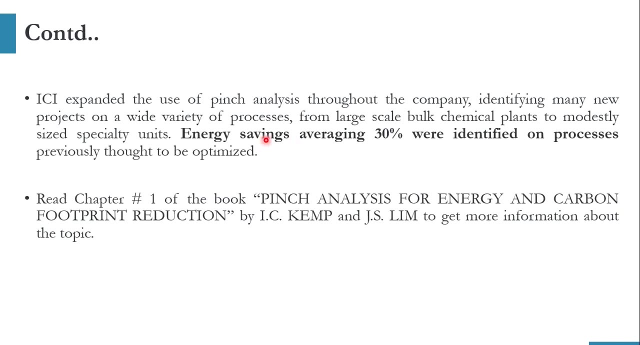 comparison to furnace, the capital cost was definitely less and even though the heat exchanger network was designed over here and even the process was further optimized and the process which was considered by the management at that time that it's a best optimized system. the optimization was done by pinch analysis and 30 percent energy savings were found in the system and that were 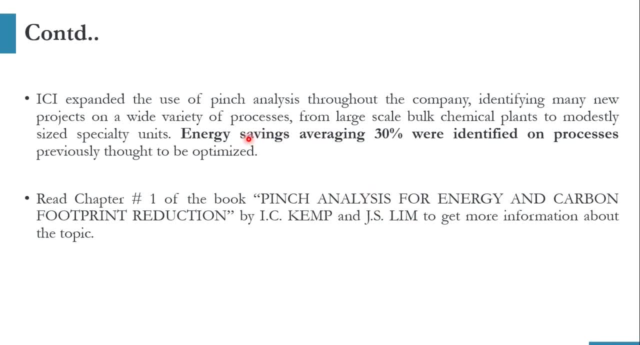 implemented. so you can see that without applying the pinch analysis, you are thinking that you have the optimized system running over here and when the team of experts came they were able to. they identified that this system is not good operated. it has a potential of 30 percent energy. 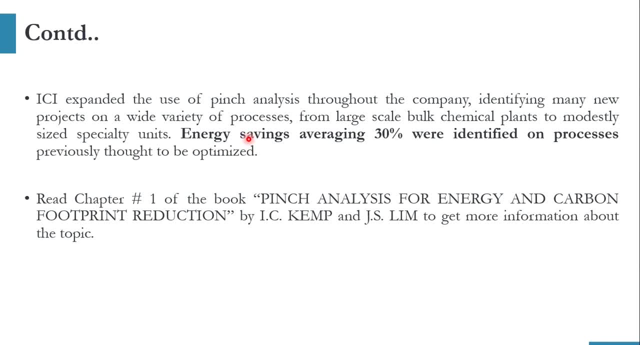 saving and if you recover the 30 percent energy saving, you can even get your 20 percent expansion within your premises. so for more information regarding the pinch analysis, you can read this book: pinch analysis for energy and carbon footprint reduction by ic camp and js slim. now why does pinch analysis work? as i have told you, its basic purpose is to optimize. 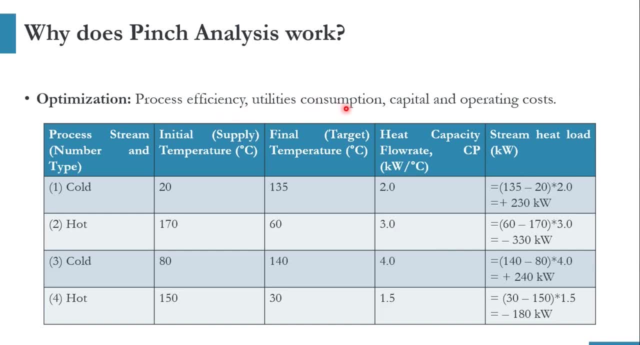 optimization means to increase the process efficiency, to decrease the utility consumption, to decrease the capital and operational cost. obviously in the previous case you have seen that you didn't require furnace, but in that case you require heat exchangers. obviously the cost for heat exchanger was definitely lower than that of the furnace. so you have four streams. the initial, 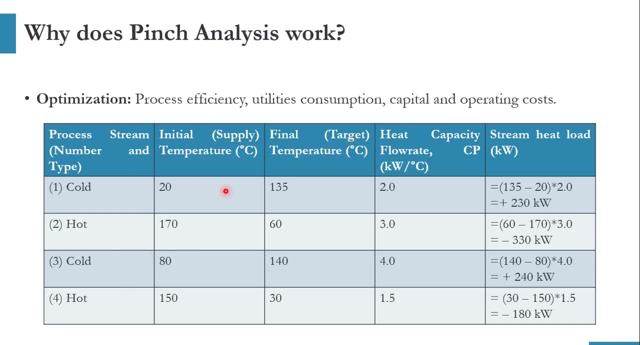 supply temperature. final target temperature. supply temperature means at which it is entering target temperature, at which it is leaving temperature and the stream. this stream is getting heat, so this is termed as a cold stream. any stream which is getting heated during the heat exchange process is known as cold. 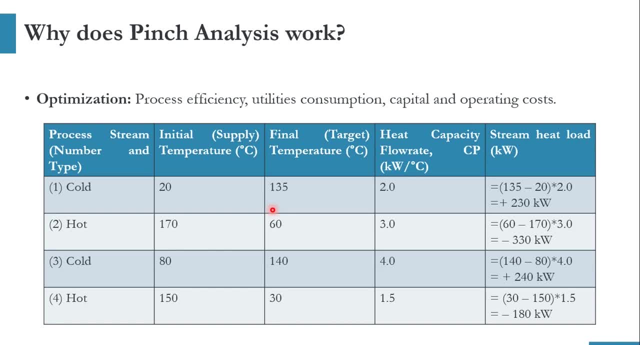 stream and the stream which loses heat during the heat exchange process is known as the hot stream. so 170 to 60 it is hot stream, 80 to 140- cold stream, 150 to 30- hot stream and this is the value of cp. i will talk about this cp in our next lecture, which is lecture. 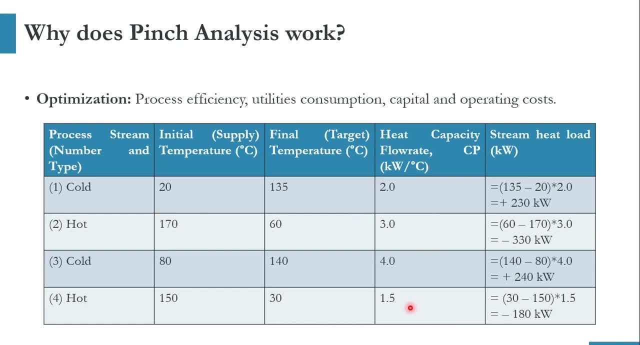 number 20.. now if you want to get the kilowatt- current unit is kilowatt over degree centigrade- obviously you need to multiply it by temperature value and currently you have two temperature values: outlet and inlet temperature. so obviously it will be calculated like outlet minus inlet. 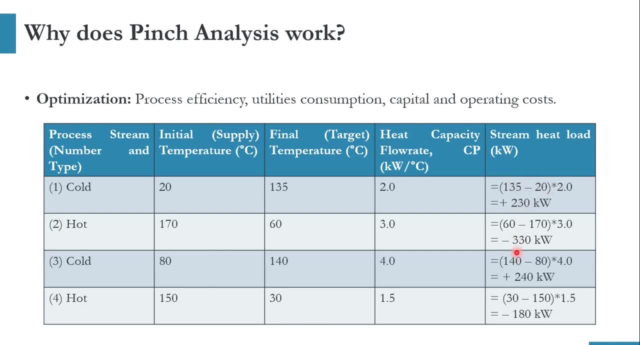 multiplied by cp. so that is plus 230 kilowatt. that is minus 330, plus 240 and minus 180- simple mathematical calculations. but now you have four streams. you want to do a heat exchanger networking. one thing is for sure from this current lecture: that pinch analysis is mainly used for heat. 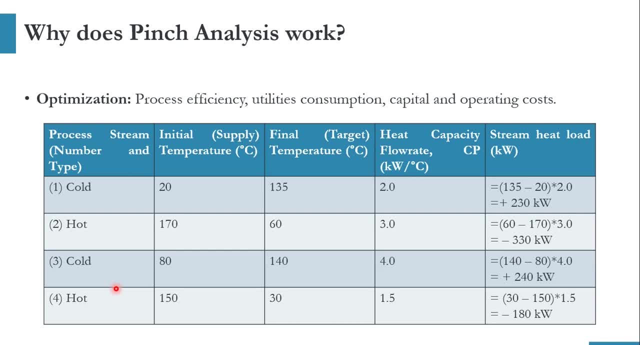 exchanger networking. that heat exchanger networking was prepared in case of ici plant. so now, if you see, do you want to match these two streams, or do you want to match these two streams, and what would be the energy requirement for this? for example, if you are using utility, you are basically required. 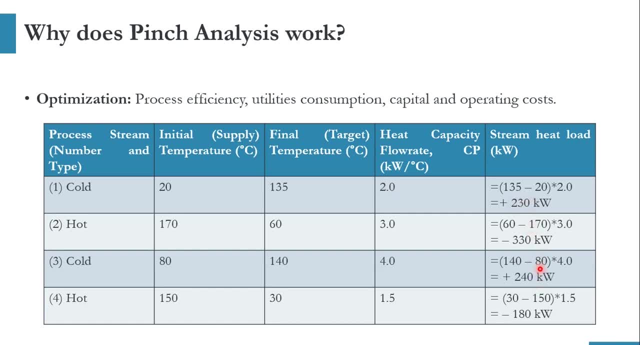 to heat these two streams. basically you need to heat these two streams: 10 kilowatt of 230 kilowatt of the heating utility, 230 plus 240, 470 to heat these two streams, and 510 kilowatt of means, second and fourth, 330 and 180, 510 kilowatt of cooling utility. but how you can decrease the cooling and heating? 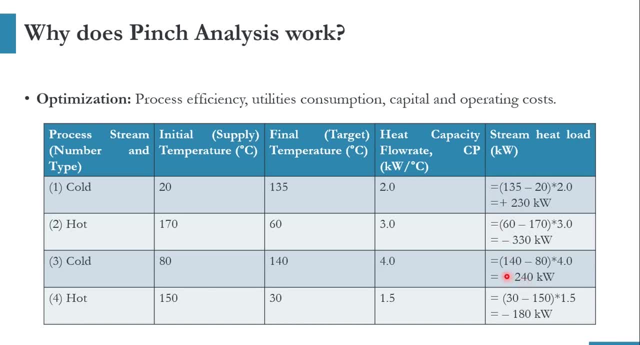 utility requirement. can you do this like hidden trial? obviously you cannot do this. you have to check the thermodynamic feasibility, you have to check that there is no temperature cross. so obviously it's not not a trivial method. it's basically a proper, established method which we have to use while 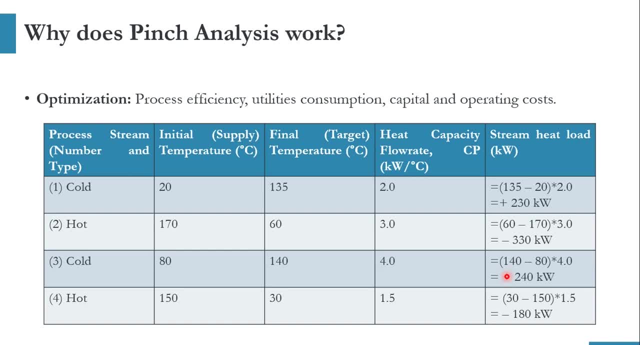 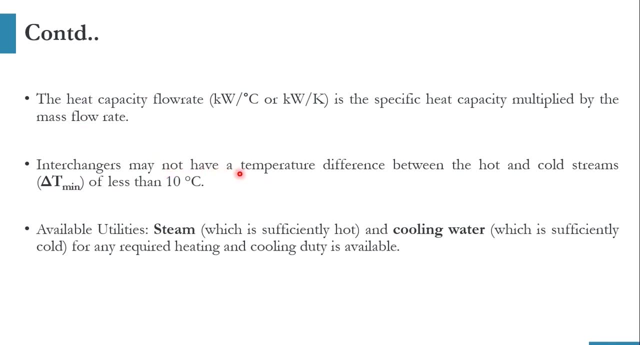 dealing with this pinch analysis and doing the heat exchanger networking. so that is also again the same, and one thing is that there the interchangers means may have not a temperature difference between hot and cold stream. this is the delta t minimum, which is usually your energy. 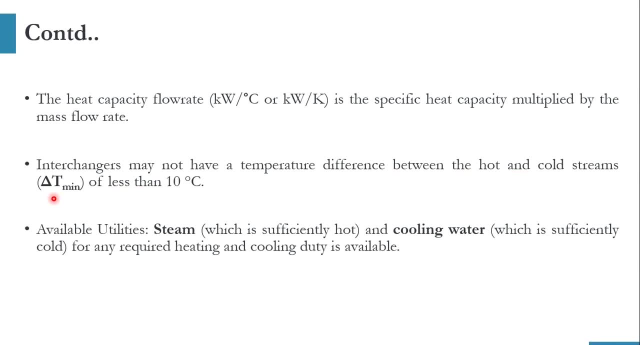 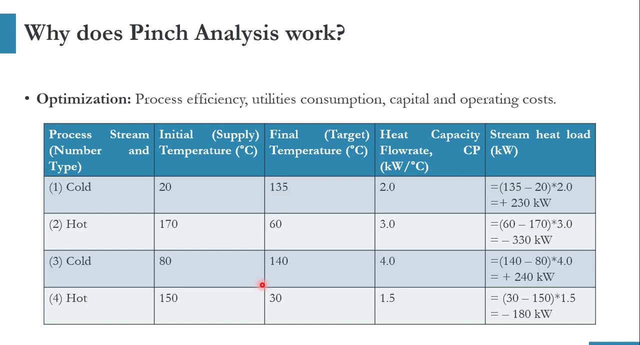 target that the minimum temperature difference between hot and cold stream at one point should not be less than, or may not be less than, 10 degree. centigrade means if i have drawn the diagram of it, or draw these lines graphically or problem table approach. these are basically. 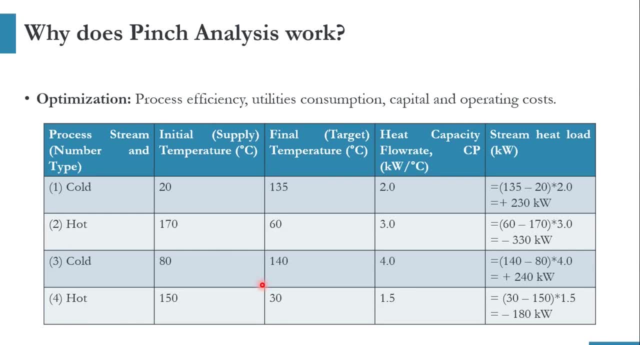 two techniques used for it, which we will talk about in our upcoming lecture, that there are two techniques for it- problem table approach and graphical method- then we will see that at each point in the interval, this may not be less than 10 degree centigrade, which is your. 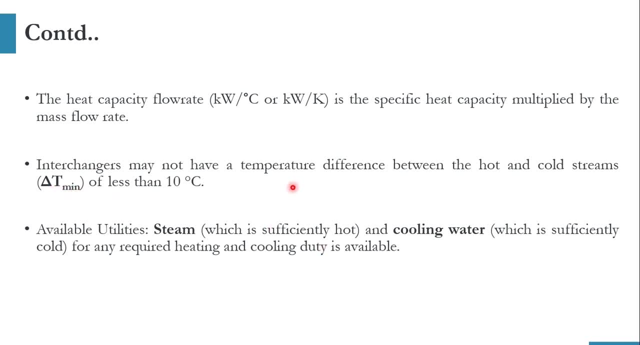 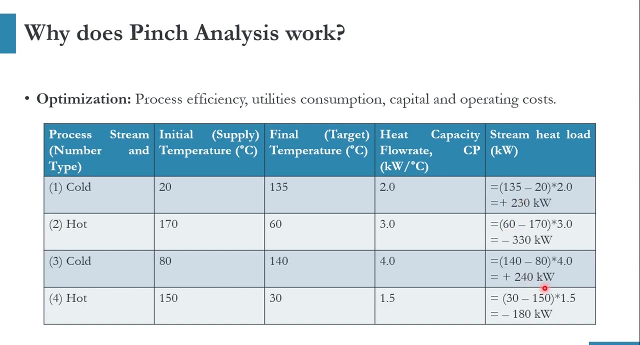 energy target, which is labeled it as delta t minimum, the temperature difference between hot streams and cold stream, but we will talk about it a bit later- and available utility: steam sufficiently hot, cooling water sufficiently cold for heating and cooling utility for this system, as i told you, 470 kilowatt steam utility is requirement, 510 kilowatt cooling water utility. 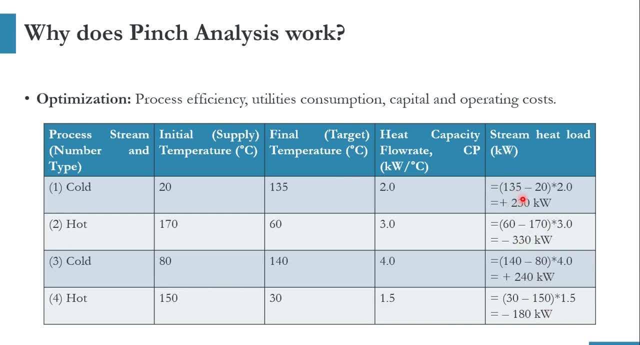 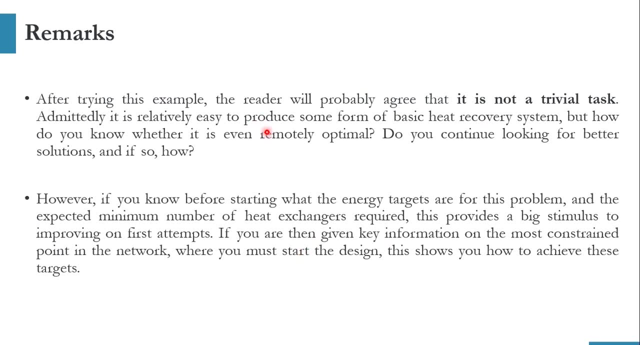 and if you want to decrease it, you cannot do it like heat and trial that connecting 230 with 330 and correcting 240 with 180 and system is solved. no, that is not the case, and this is the same point which i have already illustrated you, that it's not a trivial task. but how do you know whether? 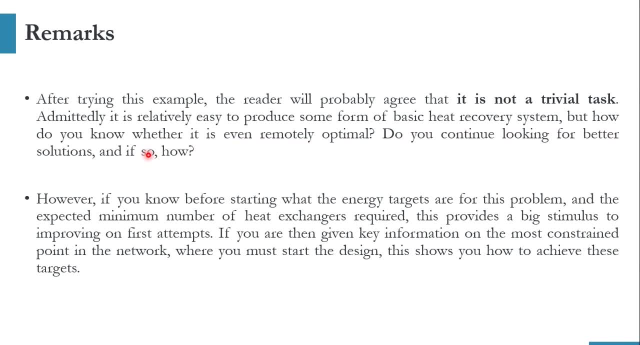 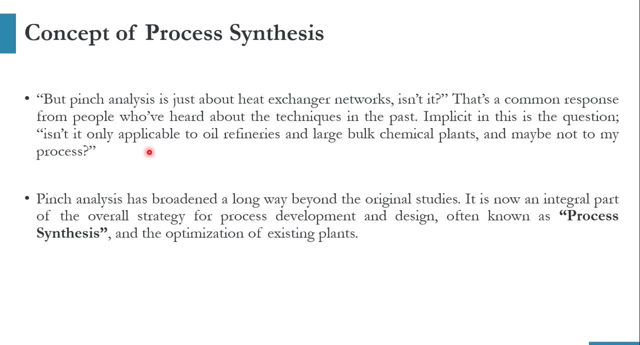 it is even remotely optimal. do you continue looking for better solution, and how? so now, once the concept was introduced in the system- and, as you can see, the concept was introduced for this, system was eliminated and heat exchanger networking was introduced. but at that time it was like: okay, so it is just about heat exchanger. networking means where heat exchanger to be. 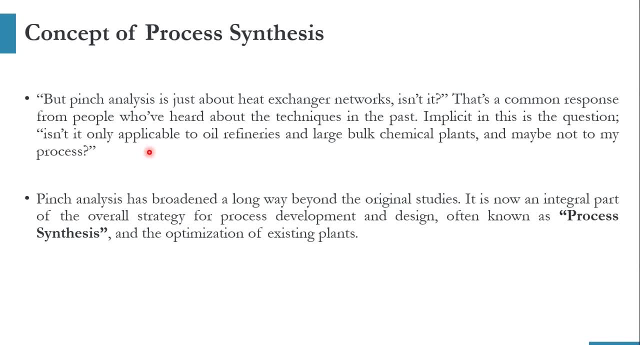 installed. it is just related to it. but it is not related to the other system. but pinch analysis is just about the heat exchange network, isn't it? that's a common response from people who have heard about the technique in the past. isn't it only applicable to oil refineries and large 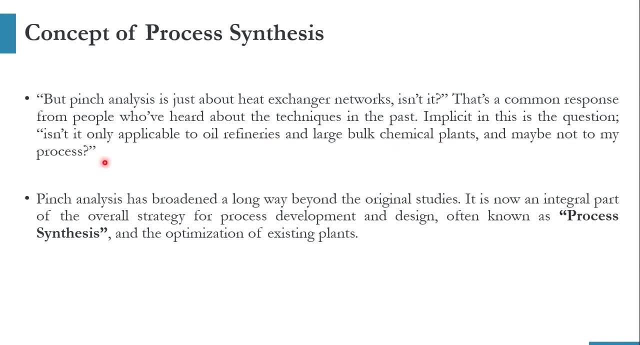 chemical plants or maybe not my process. that was another story at that time because that was oil refinery plant. so maybe, like in the fertilizer plant or in some other plant, people might be thinking, no, no, that is not applicable to my plant and that is applicable to the plant. that is definitely not the case. 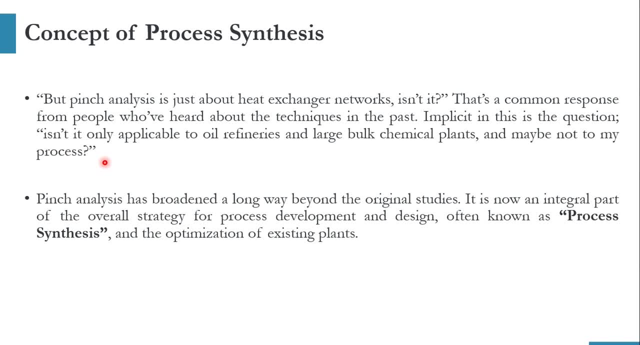 it could be applicable to each plant and each process. and obviously, where reactors are involved, the stream is going out of the reactor and it is getting heat exchange. so what do you do? you can even apply pinch analysis over there. obviously, on the reactor you cannot apply. but if a stream is, if you are sending a feed to the reactor, which? 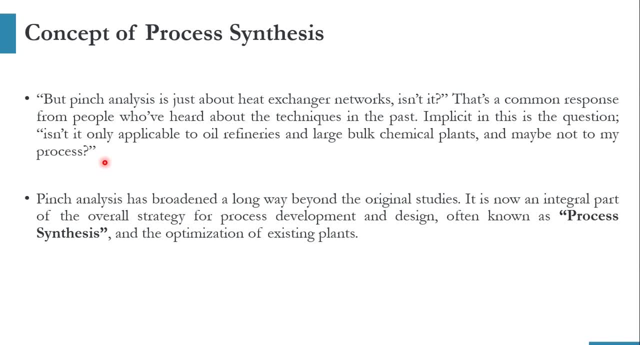 is getting heated and if you are getting product from the reactor which is getting cooled, then you can apply pinch analysis on this: that instead of cooling it down with a cooling utility you can exchange heat with the some other process in the system. but obviously with the time you will. 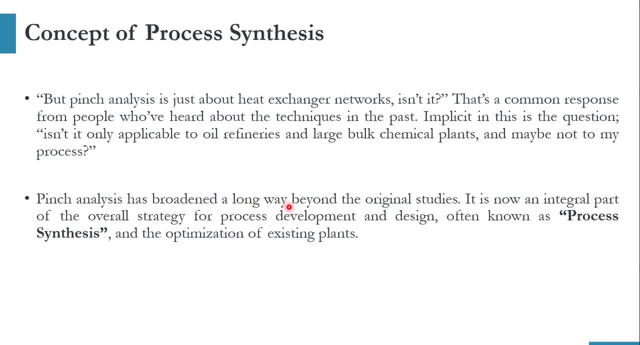 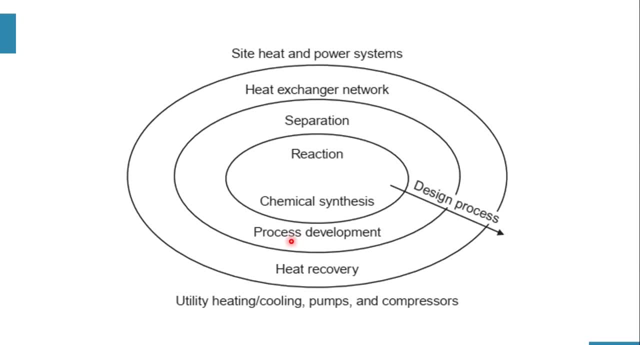 So it is an integral part of overall strategy for process development and often known as process synthesis and the optimization of existing plants. now, if you look at this diagram, there are four steps in MODENATE. first one is the reaction- chemical synthesis. obviously the process starts with the reactor. mostly in chemical industries, their first reaction takes place: the reaction. 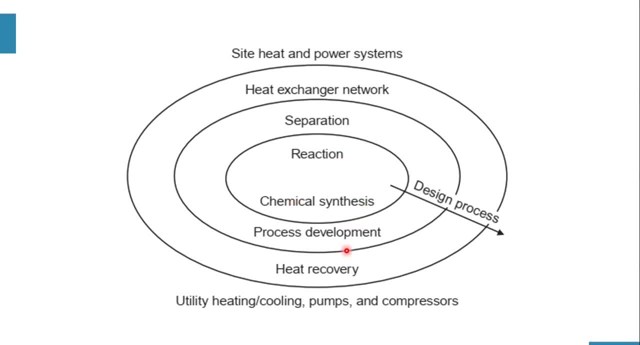 is carried out, then the separation process, development, then heat exchange. network is where you have studied the heat recovery. So you can see that even in the process where reactors, distillation columns are installed, you can even apply heat exchange and networking or pinch analysis over there as well. 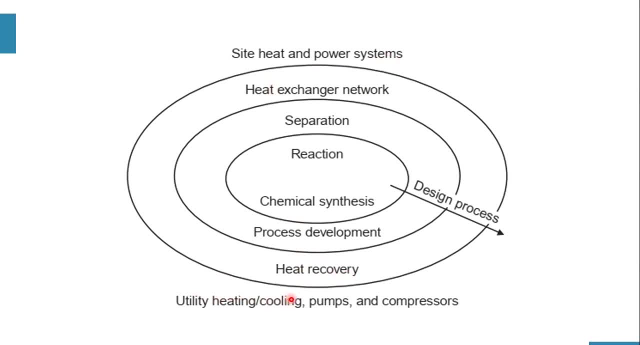 And heat recovery. and again, site heat and power system, utility cooling pumps and compressor, And you can enhance the heat recovery of the system, that you can enhance the process to process heat recovery but you can decrease the external heating requirement. So that is the overall scenario of this process, synthesis. 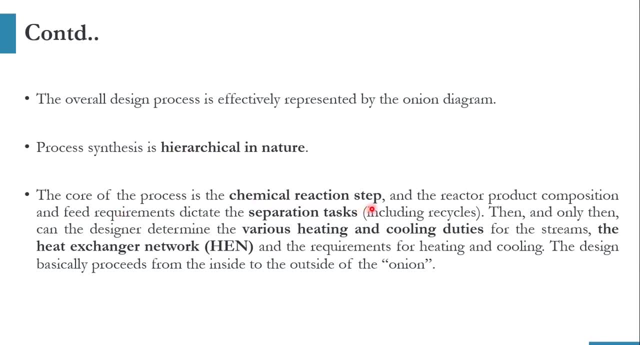 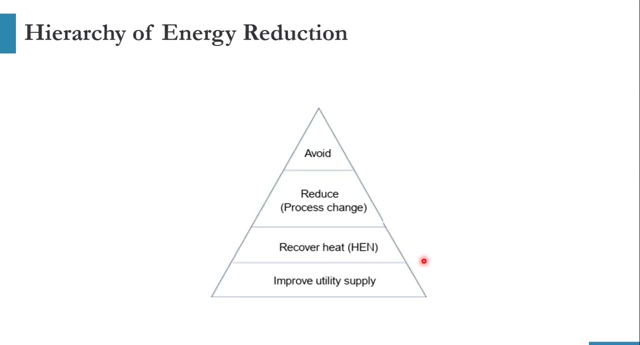 That is hierarchical in nature: chemical reaction step, then separation task, including recycles, then various heating and cooling utilities or duties for the streams, the heat exchange network, are calculated for this system. So that is overall picture of process synthesis. And the last topic of today's point is hierarchy of 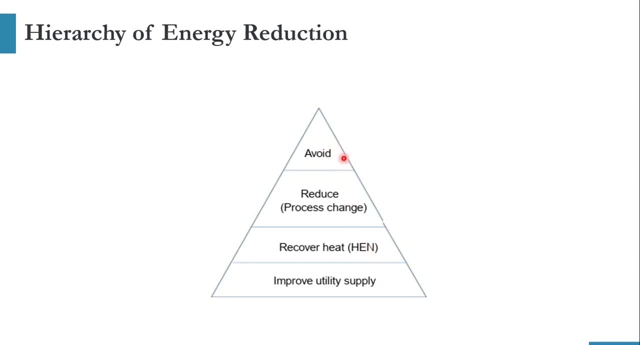 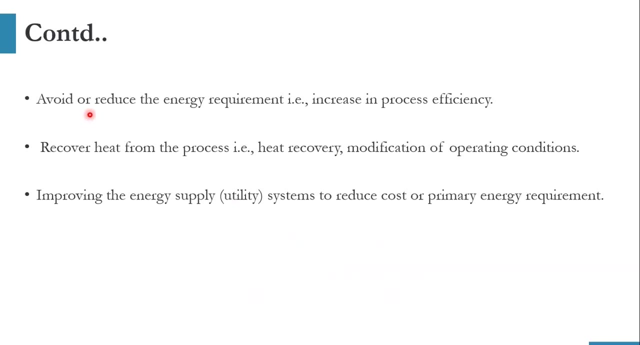 of energy reduction. The hierarchy goes from here to here: First, avoid or reduce, then recover heat and improve utility supply. Now, what is meant of it? Avoid or reduce the energy consumption? That is meant by optimization. That is meant by increasing the process efficiency. 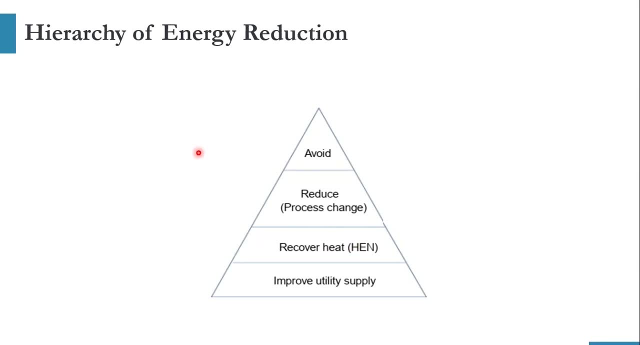 Recover heat from the process. Recover heat: It means that if a process A is releasing heat and if a process B requires heat, then integrate these two processes So that you can optimize the process. You can avoid the wastage of heat. 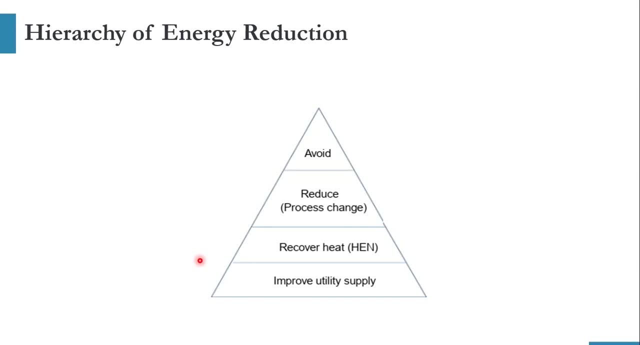 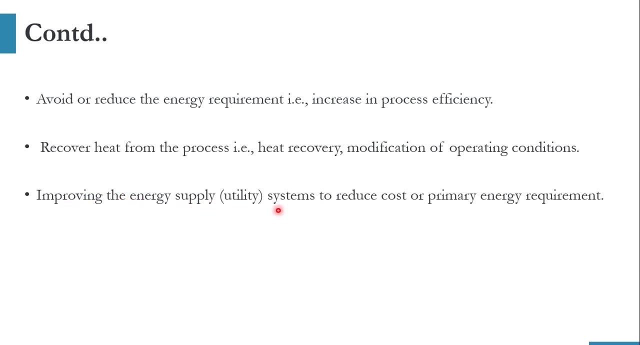 You can avoid the external utilities requirement and you can optimize the system and improving the energy supply system. And obviously, once you improve the energy supply utility system, for example, if you can run the process with steam, why are you running the process with furnace oil? 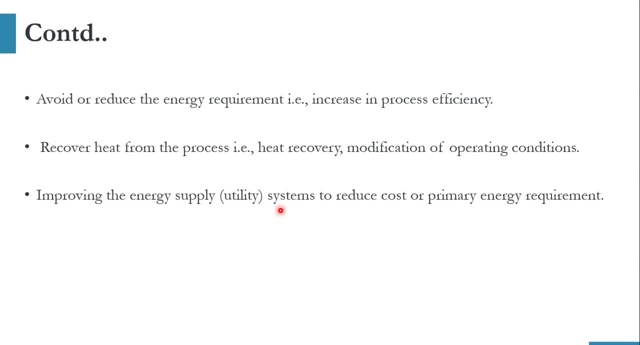 Furnace oil is obviously expensive. Similarly, if you can run the process with a cheaper utility, then why to use the expensive utility So you can reduce the cost or you can reduce the primary energy requirement. So basically the four steps. 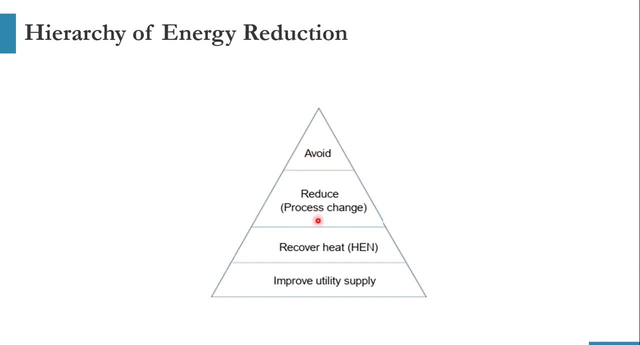 or even you can say it as three steps as well: avoid or reduce the energy consumption by analyzing the heat flows. Again, the first slide, if you remember analyzing the heat flows and determine the energy targets. Then the process inefficiencies and process improvement. 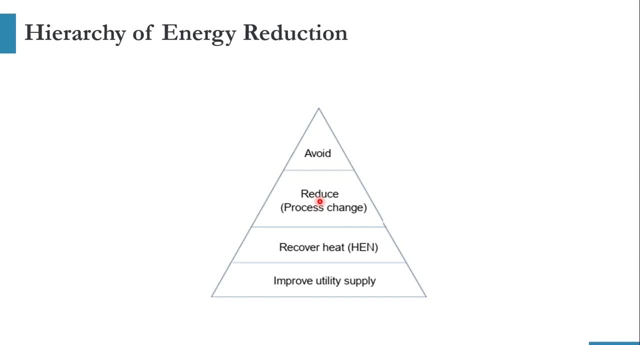 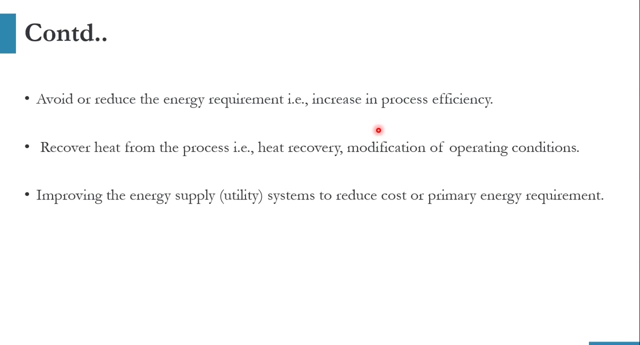 So these four, four steps are linked in our complete lecture of this session. Then recover heat and improving the utilities plan. So that's it from this lecture. Thank you so much. In the next lecture we will talk about the practical implementation of pinch analysis. 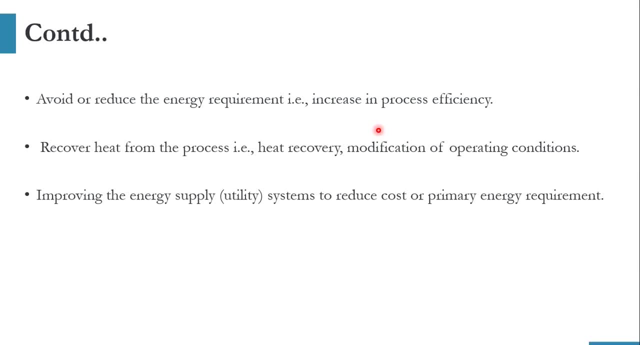 where we will use graphical method and problem table approach to find out the utilities, requirement and pinch temperatures for hot stream and cold stream. Thank you so much.